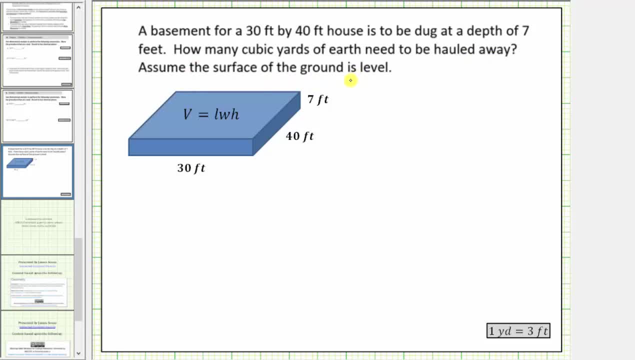 hauled away. assume the surface of the ground is level. We can model the amount of earth that needs to be hauled away using this rectangular solid where the dimensions are thirty feet by forty feet by seven feet. We will first determine the volume in cubic feet using the volume formula. 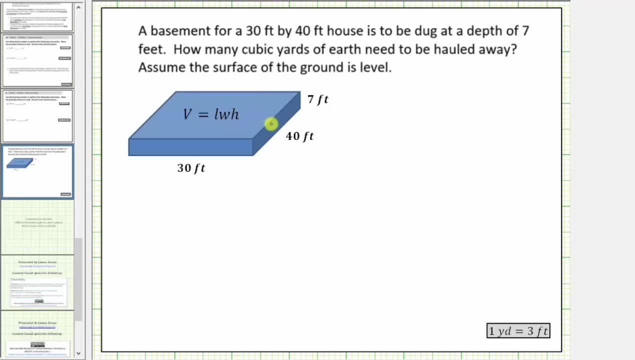 volume equals length times width times height. Then we will convert this volume to cubic yards. So the volume in cubic feet is equal to thirty feet times forty feet. times seven feet, The volume is equal to eight thousand four hundred cubic feet. And now to answer the question, we convert eight thousand four hundred cubic feet to: 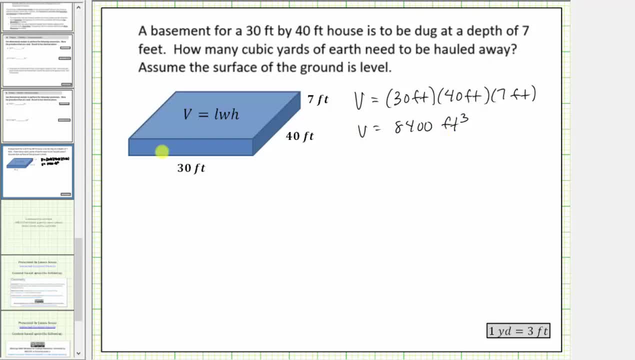 cubic yards. First, we write this volume as a fraction with a denominator of one. Next, we multiply it by a unit fraction. They will convert cubic feet to cubic yards. Because we have cubic units here, we will need three conversion factors. using the conversion, 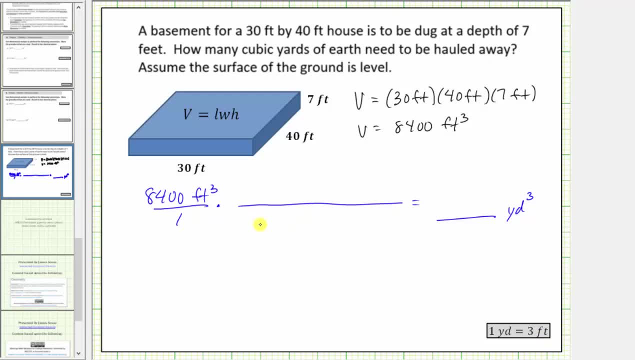 factor, One yard equals three feet. in order for feet- cubed or cubic feet- to simplify out, To begin building the unit fraction, we know we must have feet in the denominator and therefore we have yards in the numerator, Because the conversion is one yard equals. 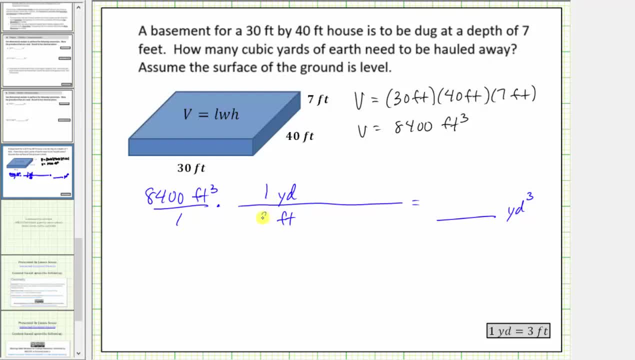 three feet. one conversion factor is one yard divided by three feet, But notice how this will not simplify out feet cubed. this will only simplify out one factor of feet. We need two more of these conversion factors to have a total of three conversion. 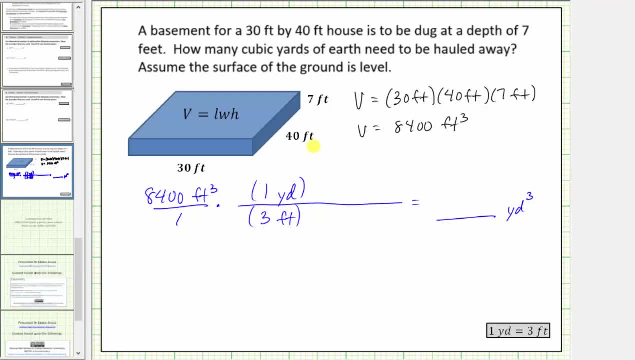 factors, so that we have feet cubed in the denominator. Notice, by forming the unit fraction with three conversion factors we now have feet cubed in the denominator as well as the numerator. So the units of feet cubed simplify to one. Also, notice how we're left with yards times.